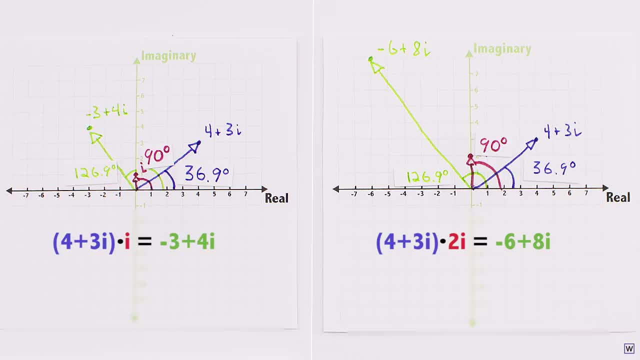 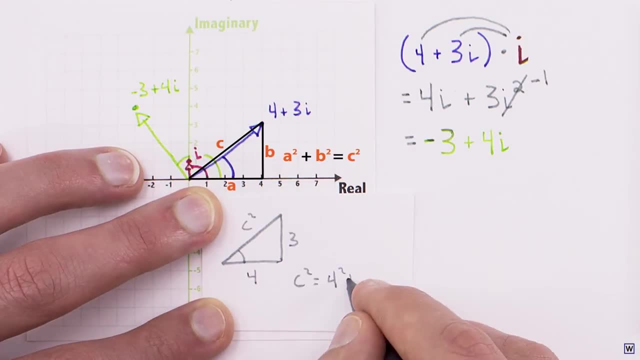 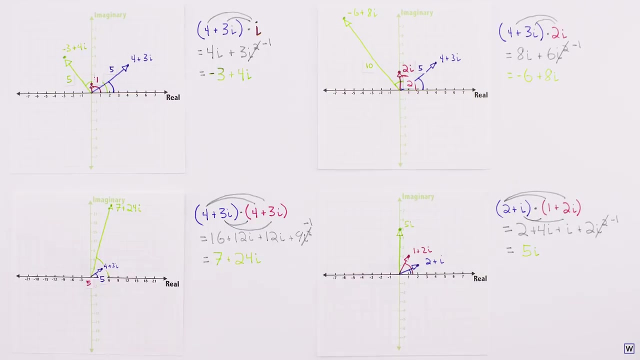 our result further from the origin than multiplying by i. A good follow-up question is how much further We can measure the distance between the origin and our complex numbers by forming right triangles and using the Pythagorean theorem. Just as before, let's compute our measurement for each example and look for patterns After. 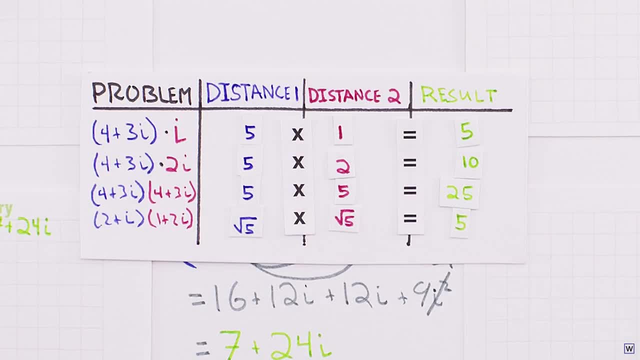 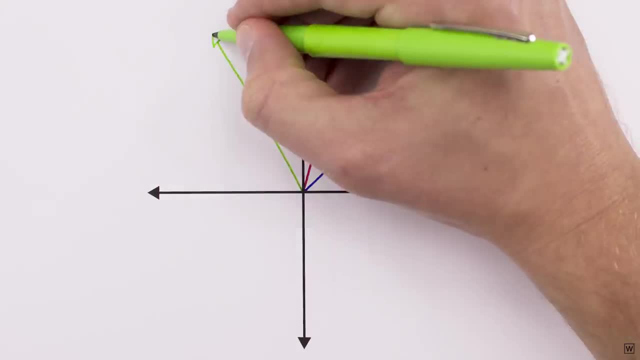 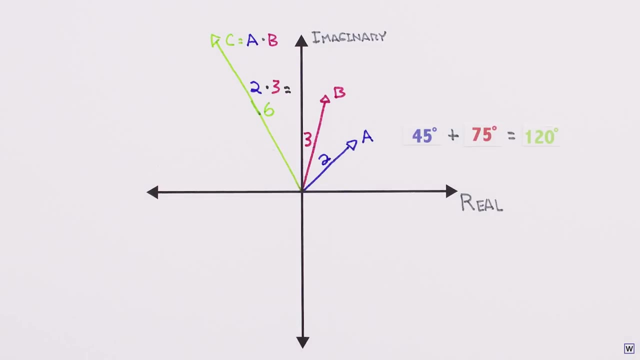 some more pondering, we see that if we multiply our distances, we obtain the distance from the origin of the result. We now have the complete picture. When we multiply complex numbers on the complex plane, their angles from the real axis add and their distances from the origin multiply. This is 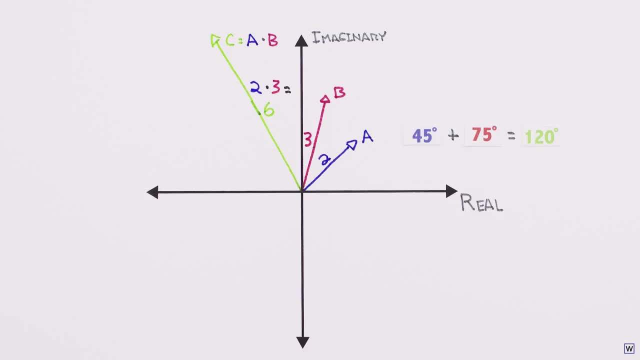 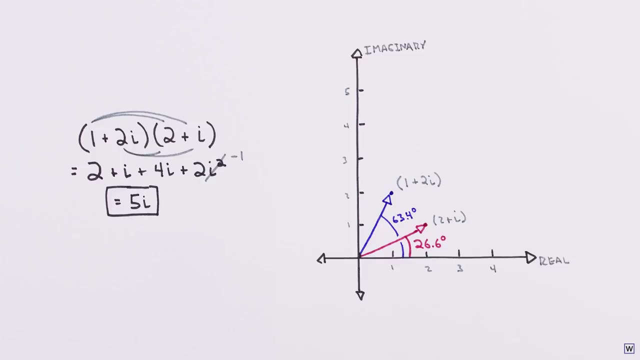 the connection we were looking for between complex multiplication and the complex plane. We now have completely separate but completely equivalent interpretations of complex multiplication. To multiply two complex numbers together, we can follow the rules of algebra or we can find each number's distance from the origin and angle to the real axis. on the complex 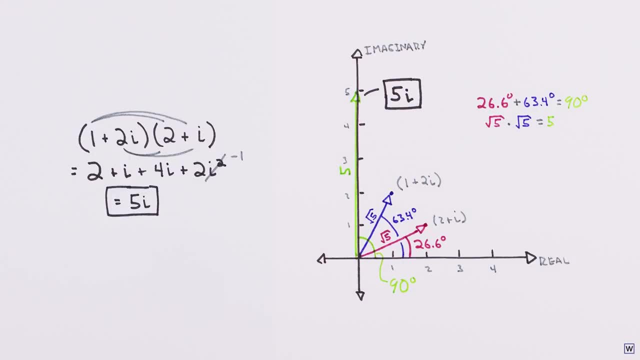 plane and multiply and add each, And what's really cool here is that, although these approaches look and are totally different, they do the same exact thing. What we're seeing here is the same underlying process from two separate vantage points. I really like this idea because it reminds me that there's more to math than what we. 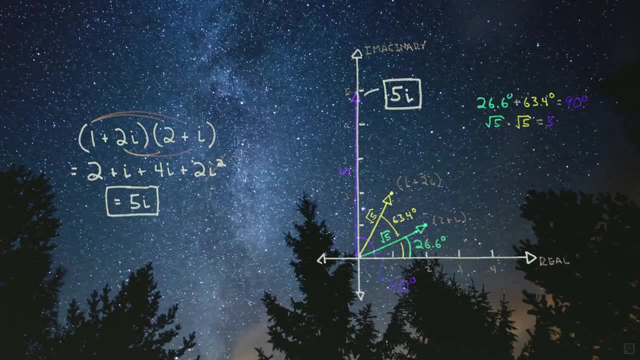 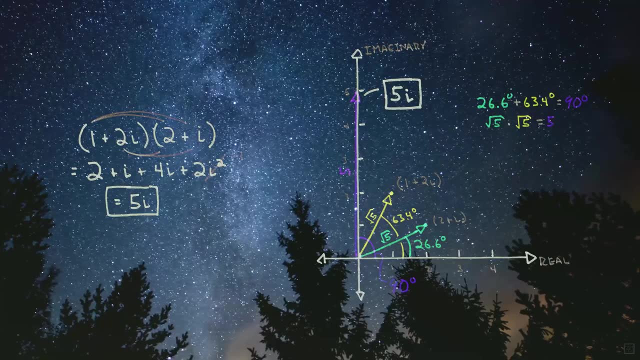 see on the page. There are deeper truths embedded in our universe, and math is one way of expressing them. Now that we've made our discovery, let's formalize our results a bit. We found that the quantities we should keep track of when multiplying complex numbers 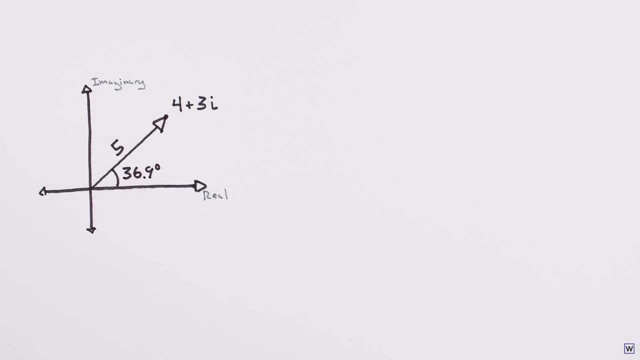 on the complex plane are the distance from the origin and the angle from the real axis. These quantities turn out to be so important that we use them as another way to write complex numbers, Instead of writing complex numbers as the sum of their real and imaginary parts. 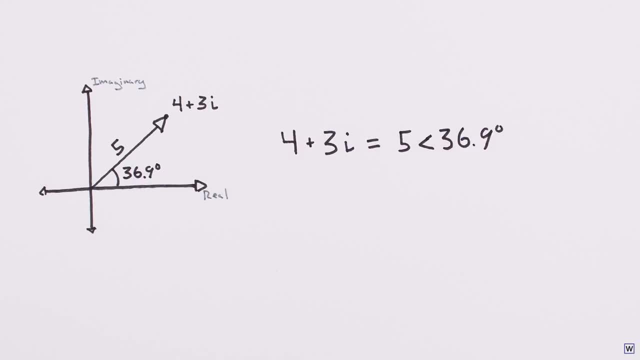 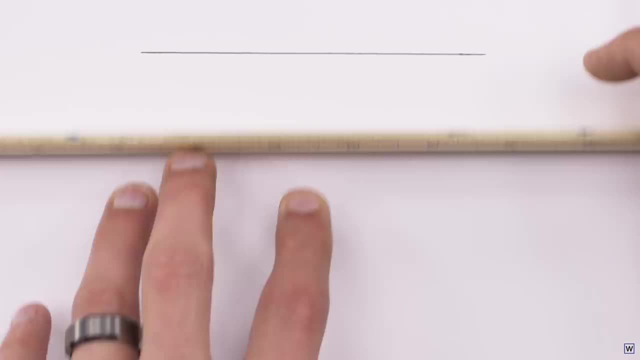 we write them as their distance from the origin and the angle they make with the real axis. This is called polar form and the distance from the origin gets a special name: magnitude. Multiplying complex numbers in polar form is super easy. We just multiply the magnitudes. 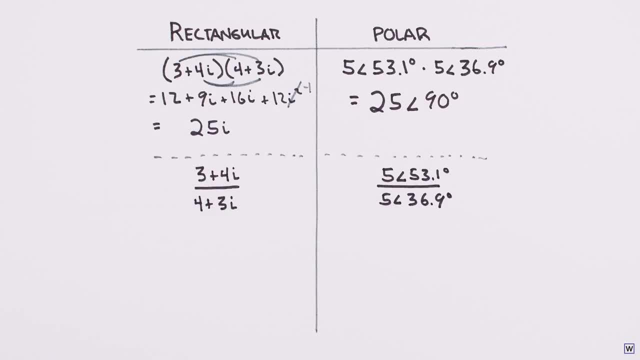 and add the angles. Division is pretty simple too, especially compared to dividing in rectangular form. To divide in polar form, we divide the magnitudes and subtract our angles. Next time we'll show that this discovery is not only cool, but also interesting.